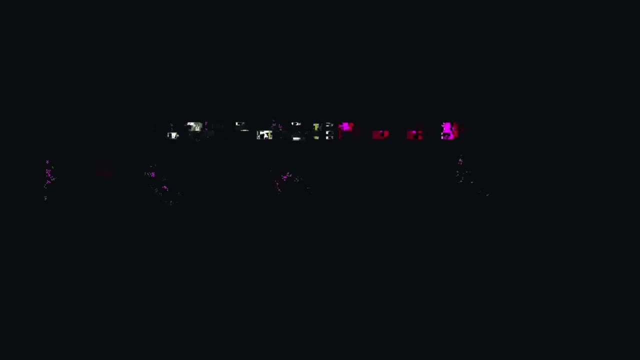 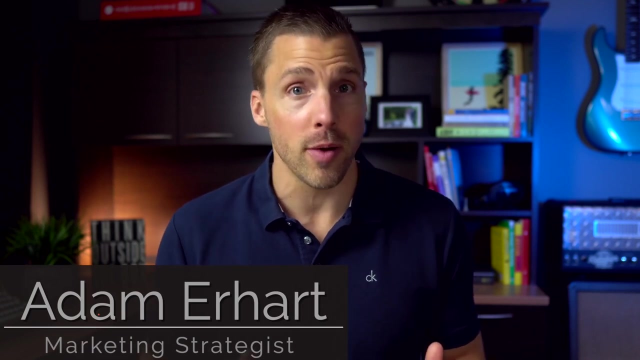 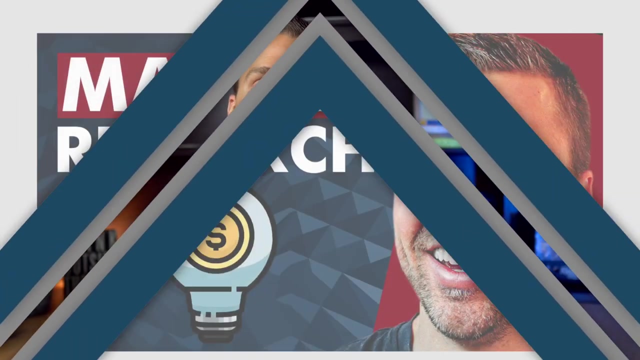 and profitable activities you can do, So let's get to it. Hey there, my name is Adam Earhart and welcome to the channel, the number one place for entrepreneurs to learn proven marketing strategies to grow their business online. All right, so let's talk market research, And I appreciate this is definitely not the sexiest. 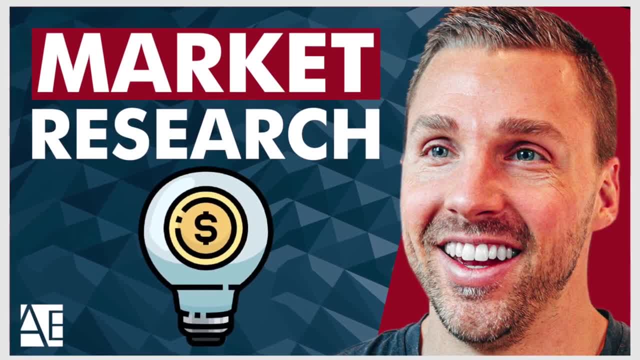 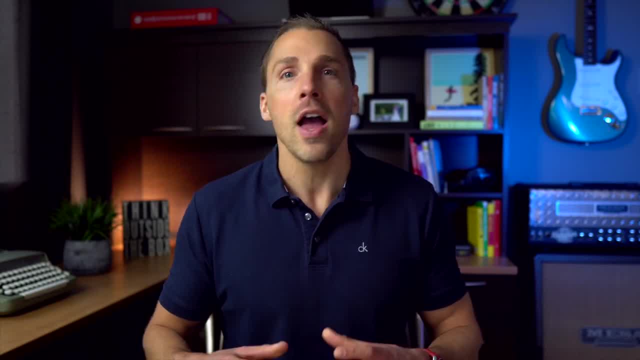 of all the topics out there. I mean. even the word research is baked right into the title, which makes it automatically sound boring. At least, that's how I used to feel until I realized the true power of really understanding your customer, their wants and their needs, and 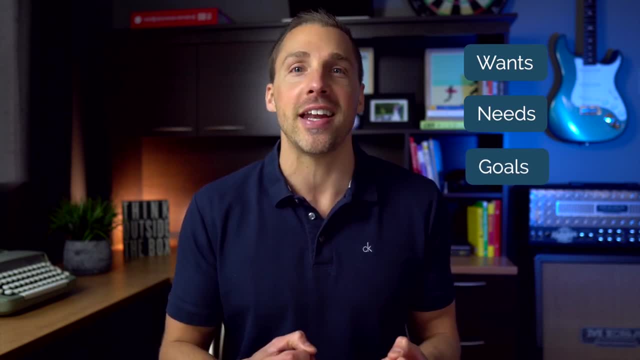 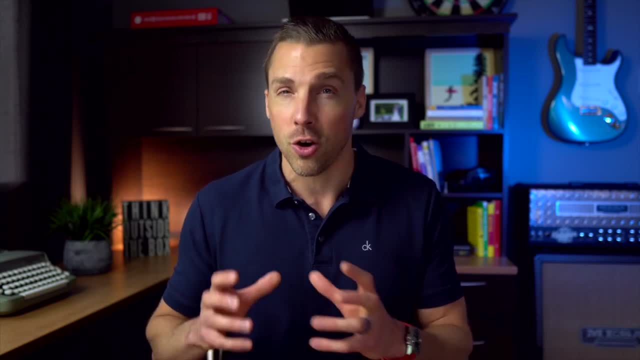 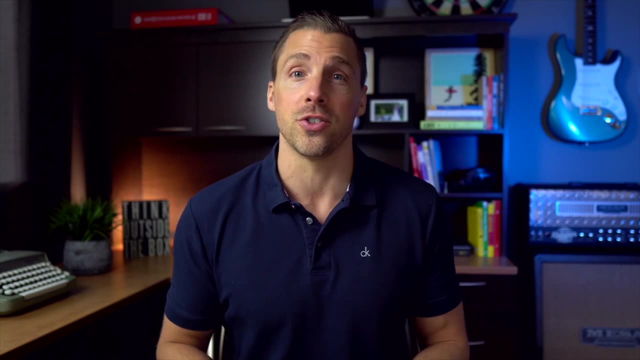 So let's get started. Let's start with the first point, which is you're going to position your business or your offer as the main, the only, the core solution to their problems, making your business kind of inevitable that it's going to be the only logical choice for your ideal target market. 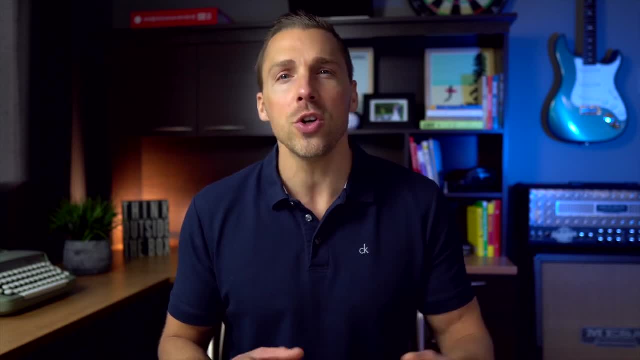 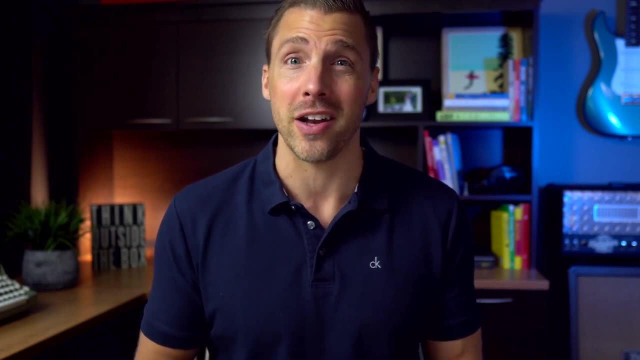 And this is hugely powerful, because if you don't understand- and I mean really understand- what your ideal target market wants, then it's really unlikely that you're going to be able to give them exactly what they want, which means they're probably going to go to your competitors. 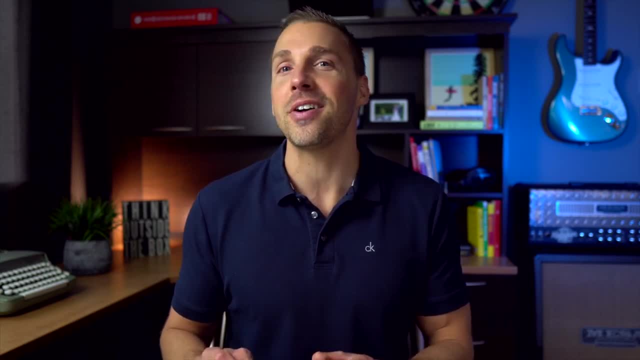 But if you understand- and you will know how to do this by the end of this video- how to uncover exactly what your ideal target market wants, it's gonna make coming up with irresistible offers almost effortless, because all you're really gonna need to do is align your offers and align what your services. 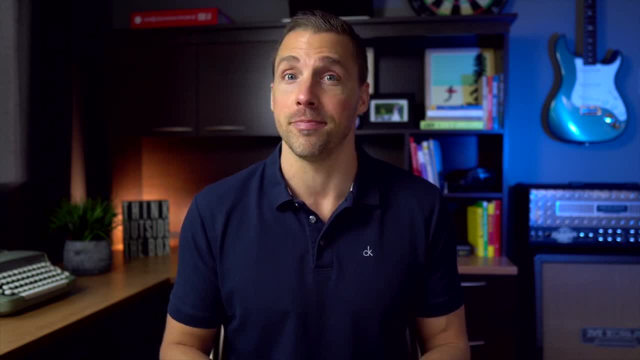 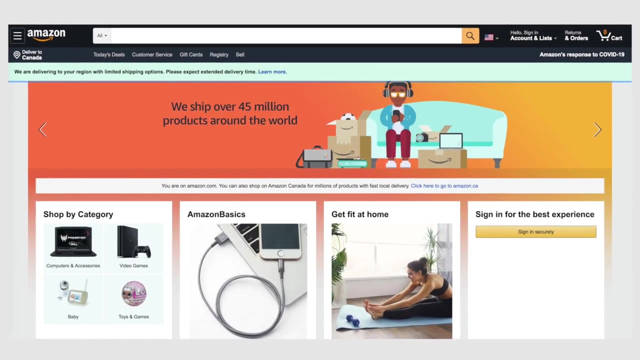 or what your products are to your customers with exactly what they want. So to figure out exactly what your customer wants, well, let's get started with Amazon Now. the reason Amazon is at the top of the list is because it is by far the fastest and the easiest way. 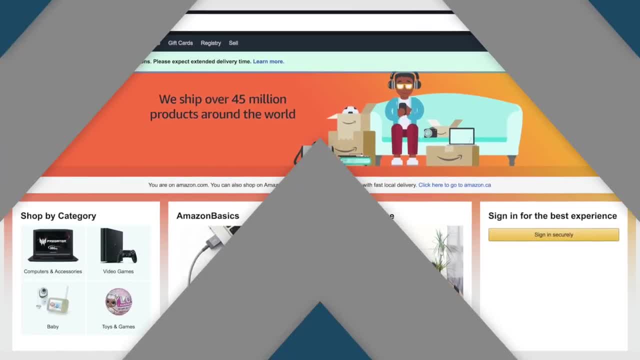 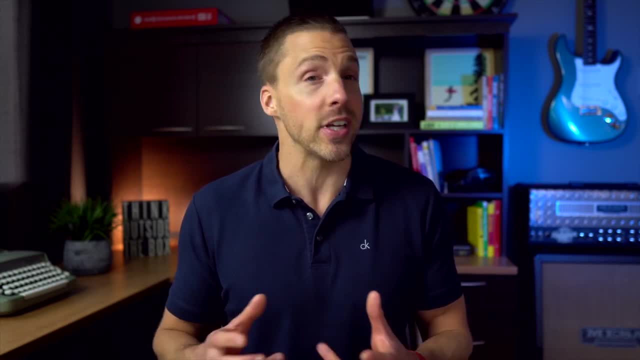 to quickly uncover pretty much exactly what your customers are thinking, what they're searching for and, most importantly, what they're actually buying. You see, one of the biggest problems with market research- at least how it's traditionally done- is that it's relying a lot on what people say. 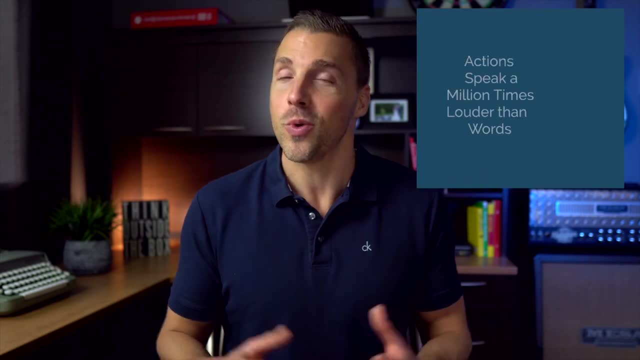 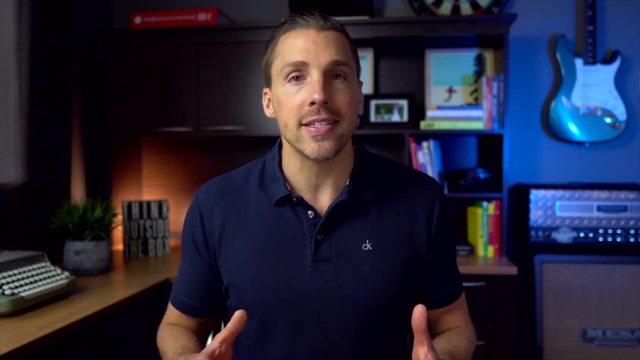 and what they say is very rarely what they actually do, which is why actions speak a million times louder than words. This is why I love heading over to Amazon to start my market research, essentially typing in my keyword and seeing what books are available on the subject. 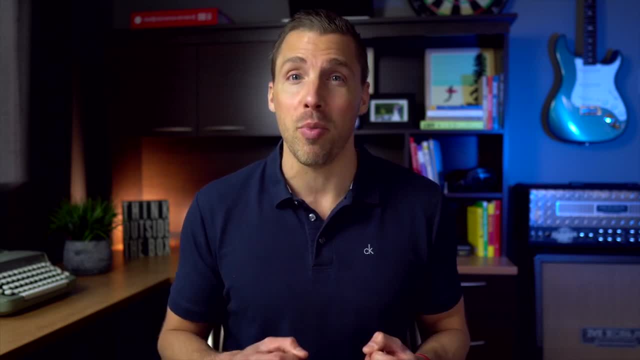 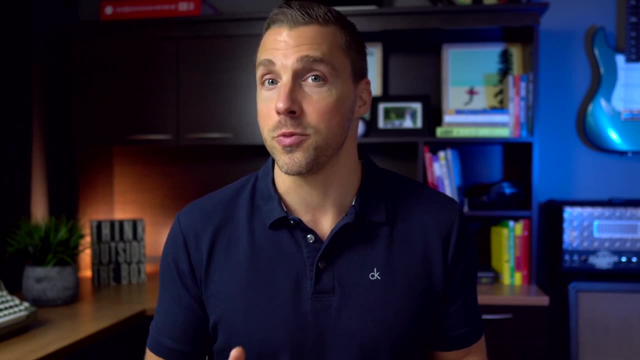 And then again, most importantly, seeing what books are actually being bought, and you can sort of judge this based on the number of reviews that they're currently getting. Other good thing about sorting out your topics and your titles based on number of reviews is that it's also gonna show you. 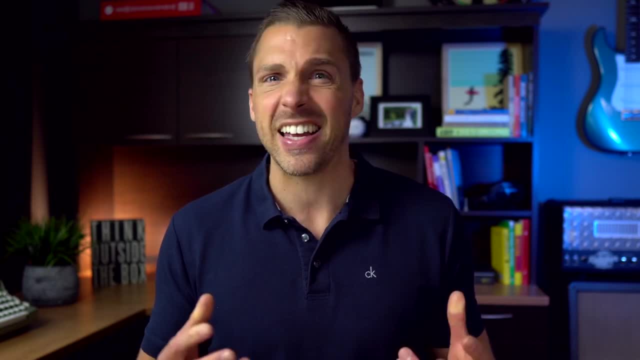 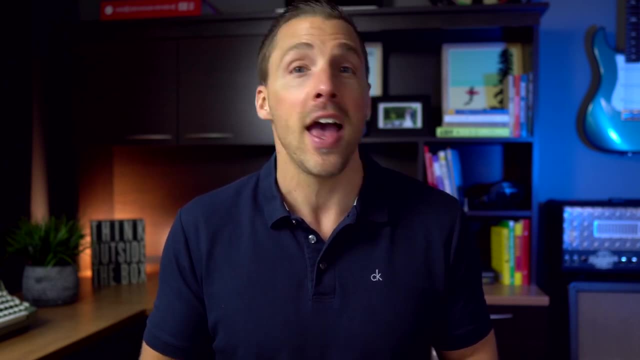 kind of the hotness of the topic or sort of the, I guess the interesting factor about like how interesting is this topic? that someone is willing to read the book and then comment on it either positively or negatively. And there's gold in both positive and negative reviews. 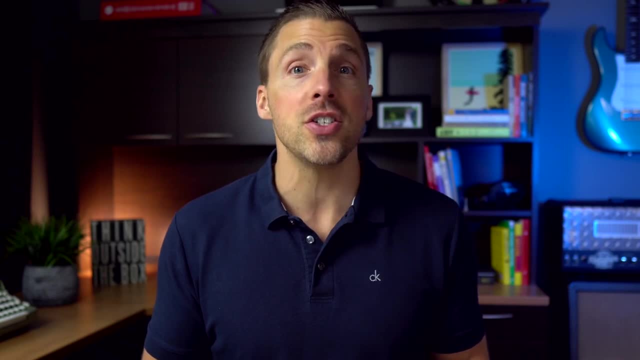 we'll get to in just a second. So the very first place to start is obviously just taking a look at the book titles themselves. Now we are taking a bit of a leap of faith here and assuming that the author did some market research themselves before they wrote the book. 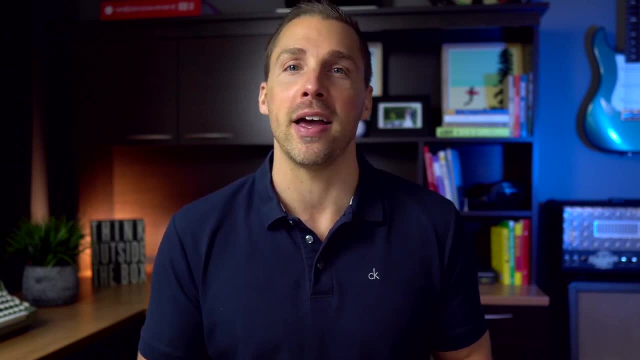 but it's probably safe to say, especially if it's an actual published book. you can buy a paperback or hard copy version of that. they probably did a little bit of due diligence and they did come up with a relatively strategic title in alignment with their target market. 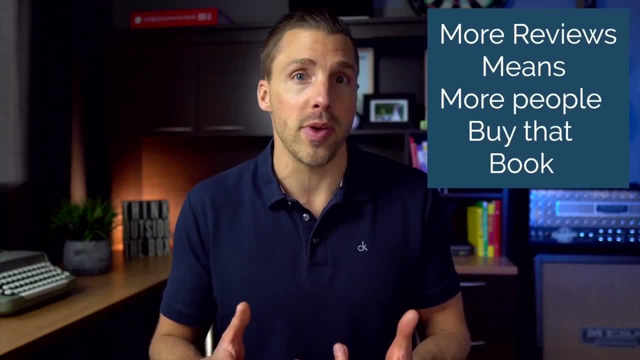 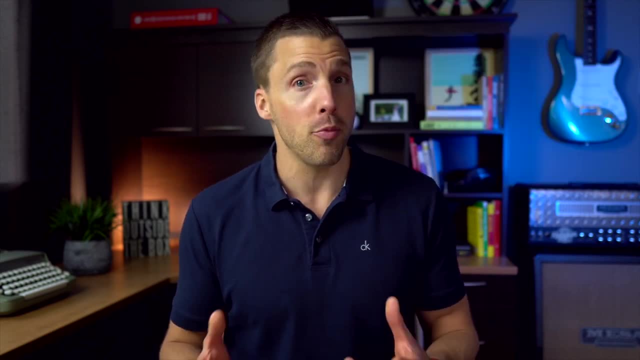 From there you wanna take a look at the reviews. Obviously, the more reviews well, the more people probably consumed the book and, more importantly, that we're interested in or engaged enough to leave some kind of a content, Both positive and negative reviews. 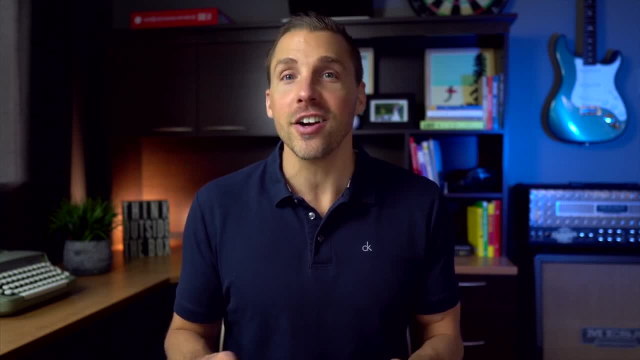 are gonna be helpful here. The positive reviews are fantastic because they're gonna tell us exactly why readers thought this book was valuable, what their most interesting takeaways were, what the lessons were, how it helped them. maybe some stories or some examples of how they applied it in their own lives. All of this is a goldmine, But the negative reviews are just as useful because they're gonna tell us all the places that the book missed the mark. Maybe the reader had a problem that wasn't addressed? was insufficient detail in another area? Well, this leaves the door wide open for you. 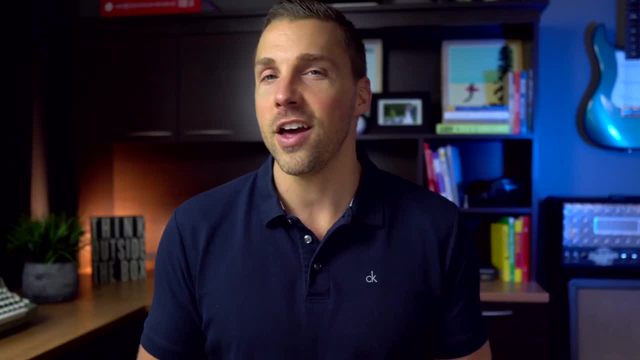 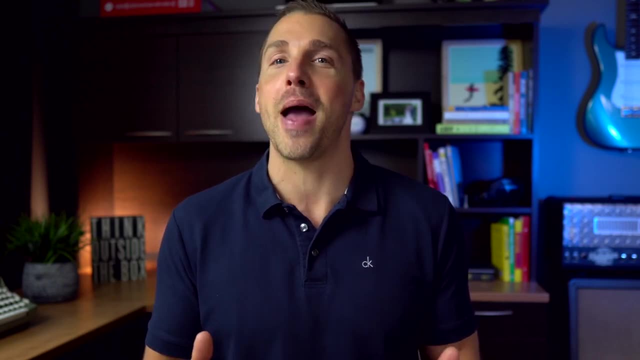 to walk through and essentially solve that problem for the readers. The other beautiful thing about Amazon is that it's pretty much ubiquitous. Like everybody knows about Amazon, Most people have purchased something from Amazon. In fact, if you've bought a book from Amazon, 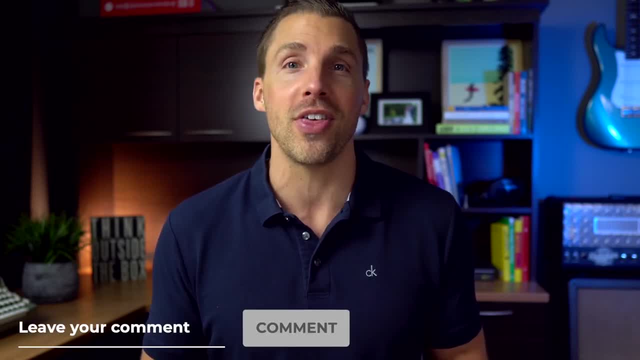 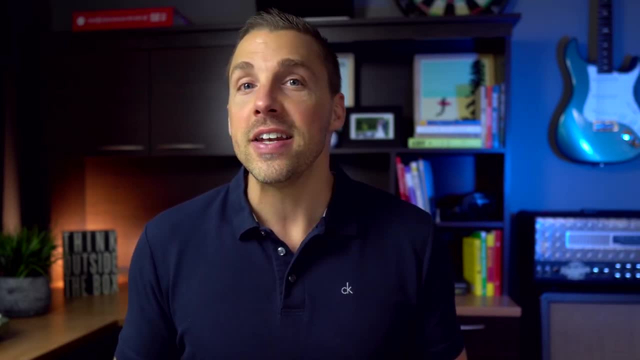 in the last year. just let me know in the comments section below what book that was And you'll start to see really quickly just how popular Amazon really is. But let me know, really curious to hear. All right, the next tool that I'd like to suggest. 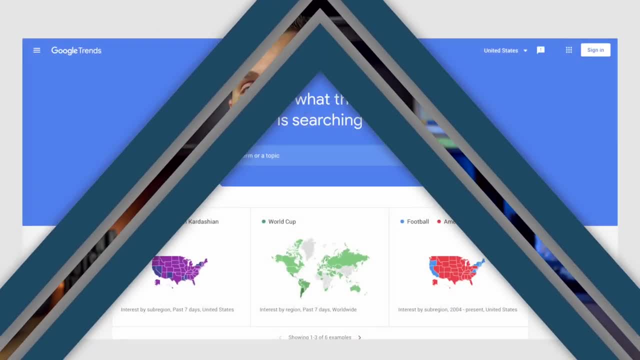 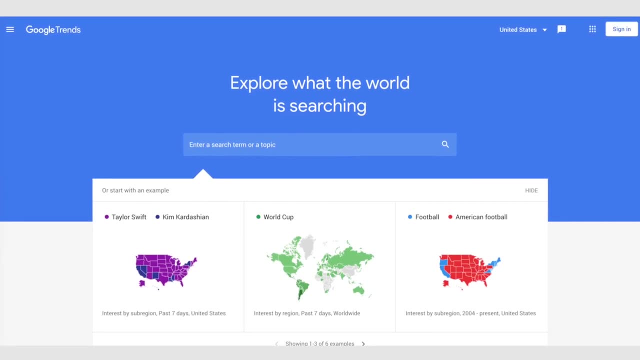 you take a look at, that's both fast and free and easy, is Google Trends. Now, obviously, Amazon is one massive behemoth of data, but another massive behemoth of data is Google. Now, Google Trends is an amazing tool, especially to get that really high level. 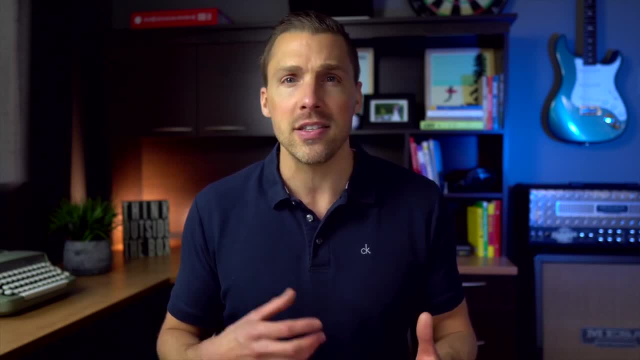 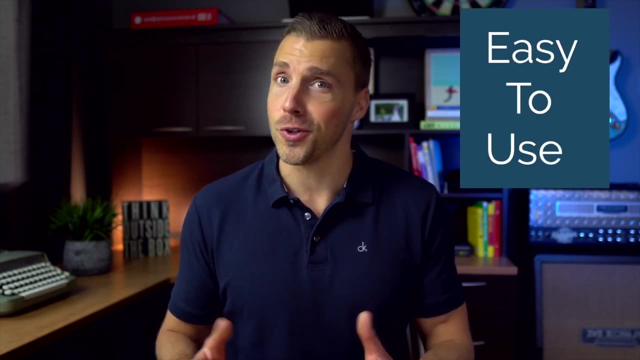 30,000 foot overview about your market and about different trends and keywords and what's popular and which direction things are going. Also, Google Trends is incredibly easy to use. You just have to search for Google Trends, Then, once you're there, you just type in your keyword. 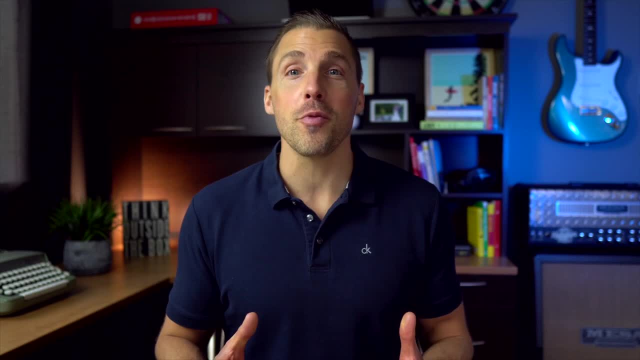 and you're presented with a ton of information. You can take this information and you can break it down based on country and based on state, based on different timelines. Beauty of this is it allows you to see if your current market or your current topic. 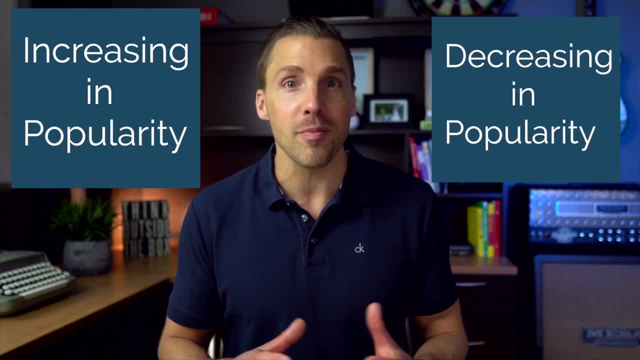 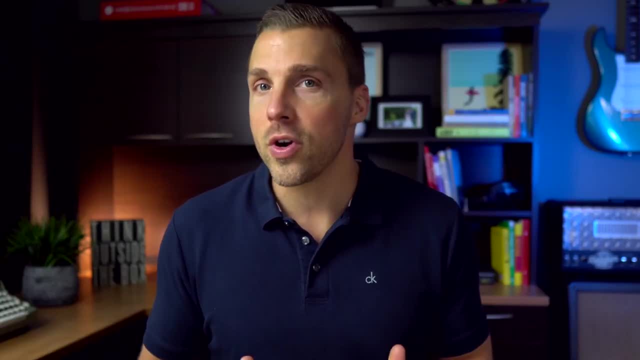 that you're searching is either growing in popularity or decreasing in popularity, or staying flat in popularity or, importantly, if there's different spikes throughout different times of the year. Google Trends will also provide you with related topics and related searches to give you even more content ideas. 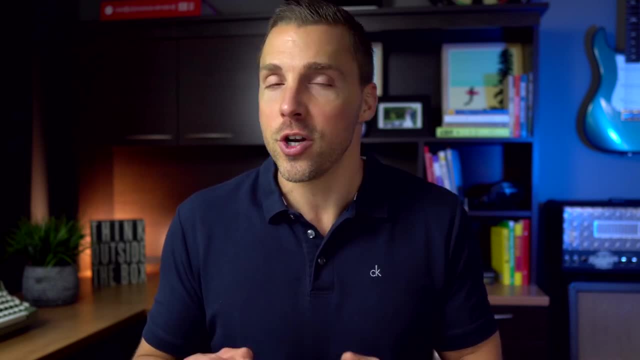 So really, between Amazon and between Google Trends, you're gonna be off to a really really good start and both free, both easy. But that's not enough and it shouldn't be right, Because you really wanna dive deep into your customer's psychology. 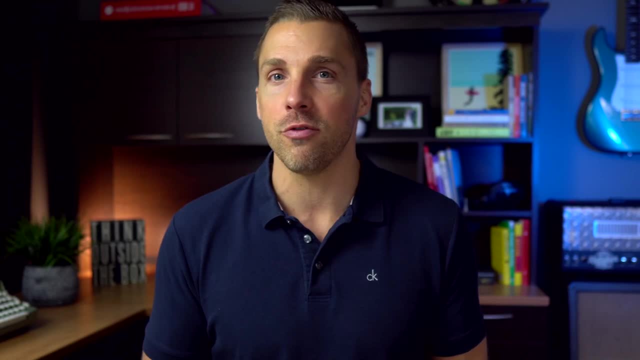 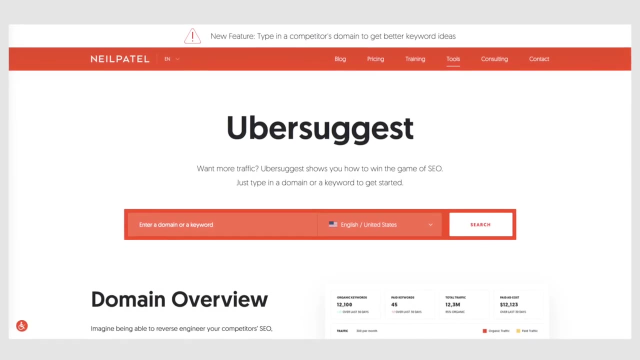 into their mindset and into their actual behaviors, what they're looking for and what they're buying. This is why one of the other tools that I absolutely love is something called Ubersuggest. Ubersuggest is both a free tool and a paid tool. 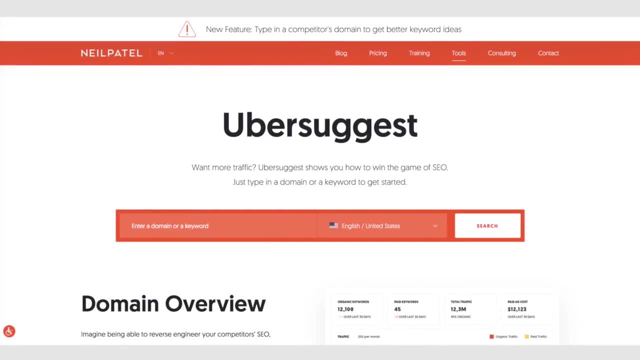 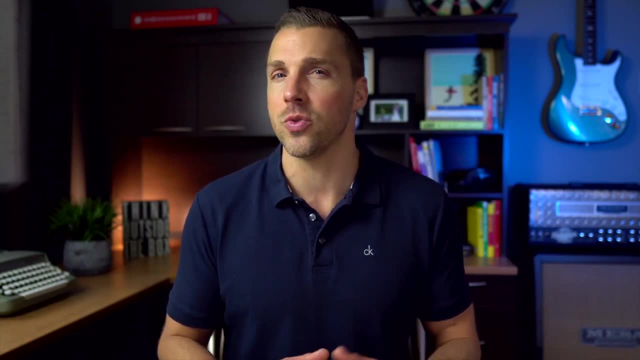 if you wanna upgrade, but definitely just get started with the free version and you'll see just how powerful it is. What it allows you to do is do some really deep, deep keyword research into your topic and into the niche that you really wanna dive into. 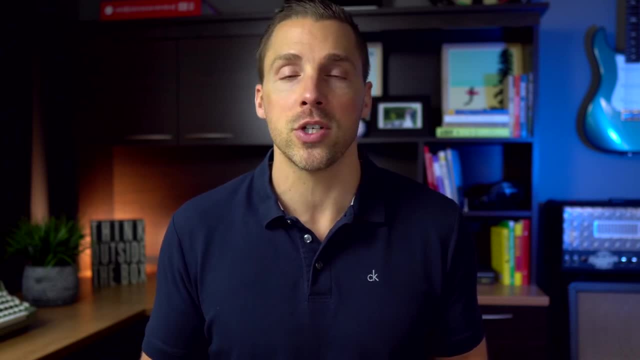 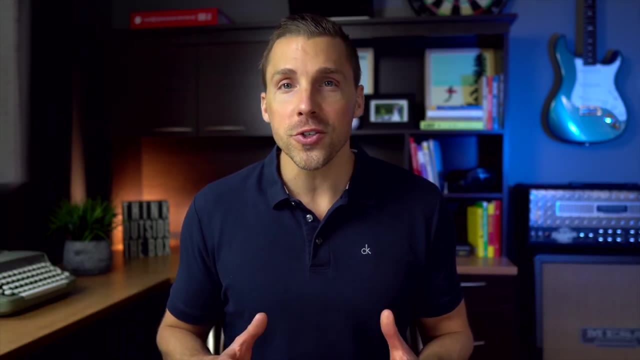 For starters, it allows you to see total search volume on the keyword, which basically shows how many people are actively searching for the topic that you wanna talk about, or for your market, or for your industry. You can also see the competitive ranking of the keyword. 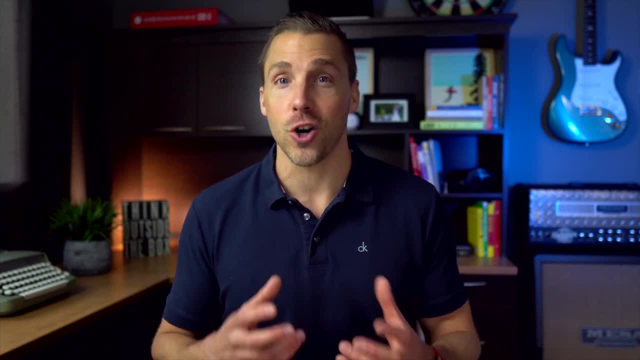 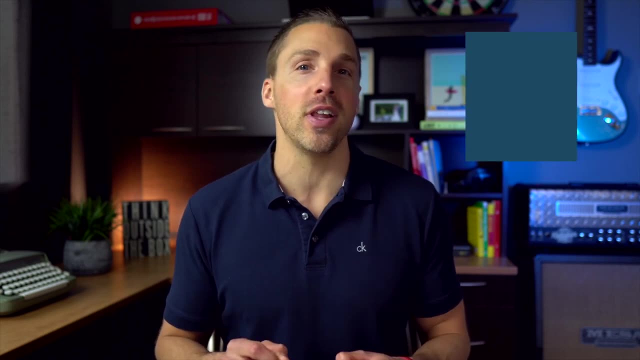 which is going to allow you to really discover well how many of your competitors are trying to go out there and capture this keyword, or capture this market as well. One of my favorite things, though, is that it shows you the cost per click, or estimated CPC. 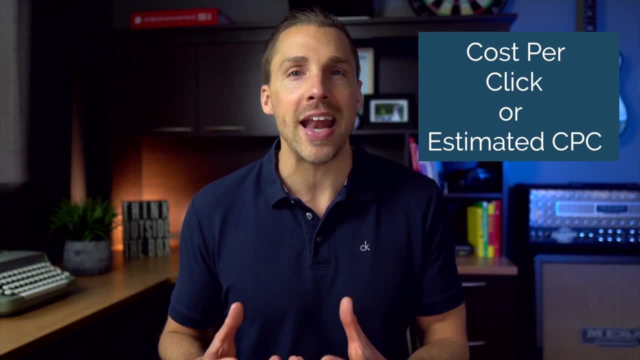 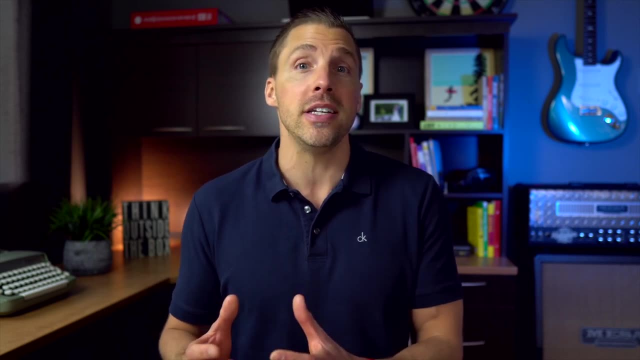 of just how much it's gonna cost you if you were to run an ad against this keyword, which allows you again to see: all right, if I wanna run ads for my market or for my business, this is what I'm gonna need to spend per click. 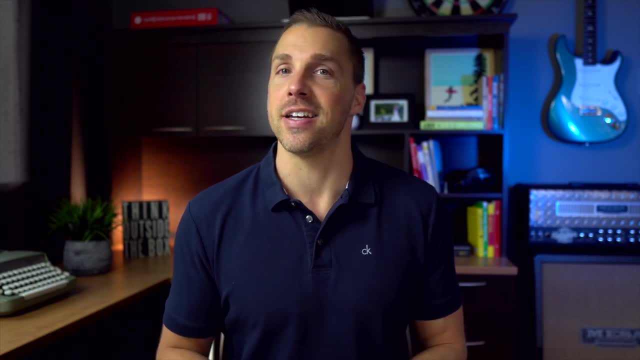 Plus, if you keep scrolling down, it'll give you additional keyword and additional content ideas, So definitely worth checking out. All right, moving right along to customer database mining. Now, if you already have a business and you've already got a customer list, 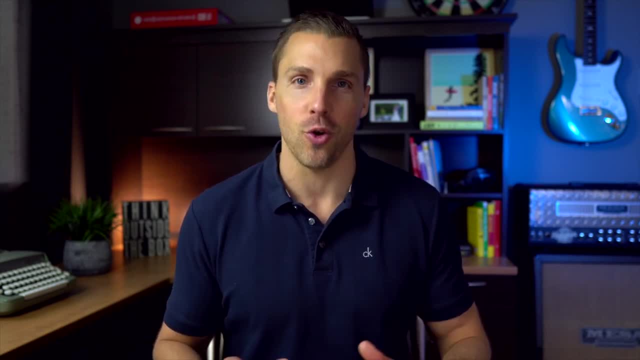 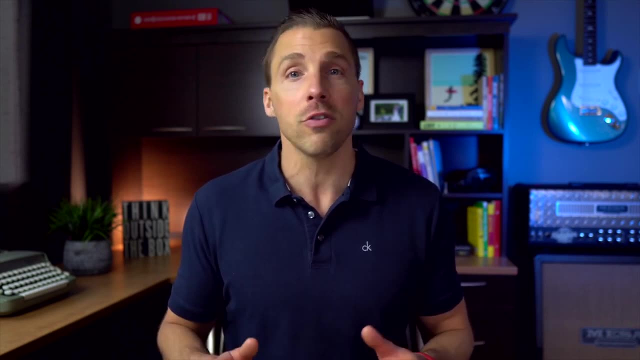 then you are sitting on the absolute target market research gold mine. Essentially, what you wanna do here is you wanna go through your customer database and you want to arrange your customers in order from least profitable all the way up to most profitable. From there, what you wanna do 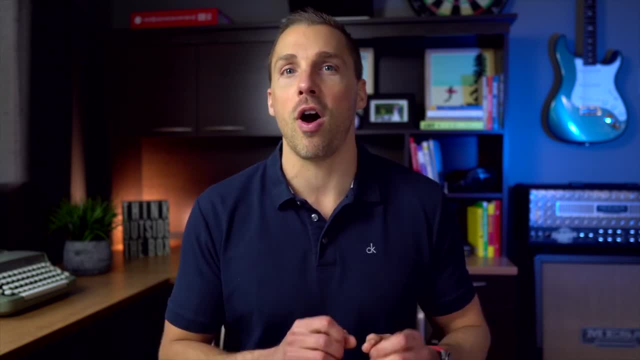 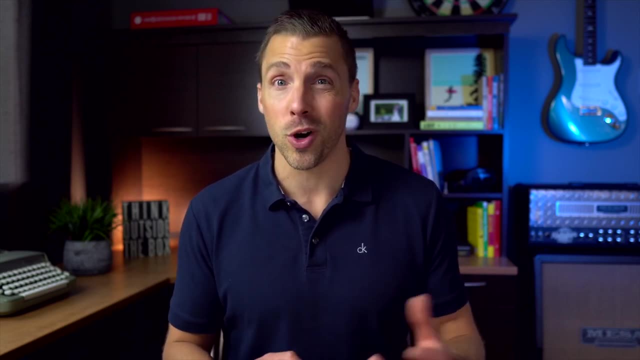 is you wanna really focus on that top 20% of your most profitable customers? These are the ones that are providing the most revenue or the most profit for your business. but also keep in mind how fun they are to work with and how enjoyable it is to deliver the service. 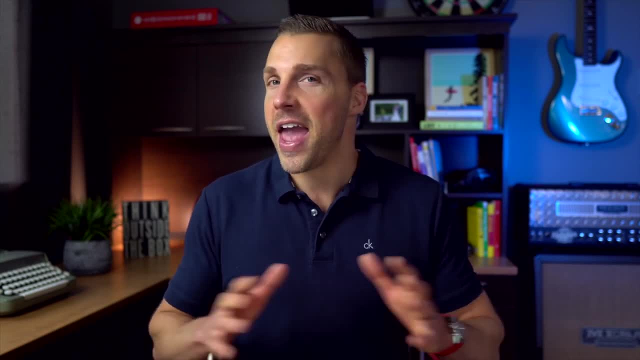 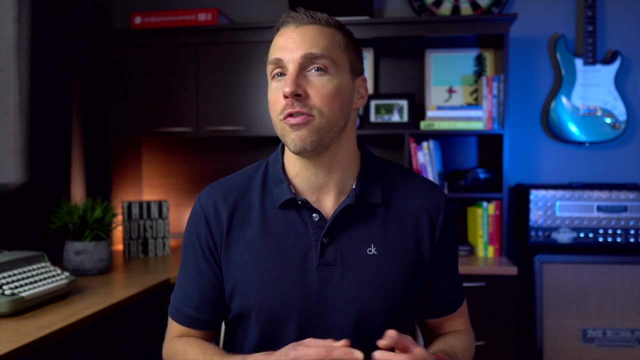 for this group of customers. Once you've got this group, you've 80-20-ed your list, essentially run the Pareto's principle against your customers. well, you wanna focus on that top 20% and you wanna look for common themes and characteristics. 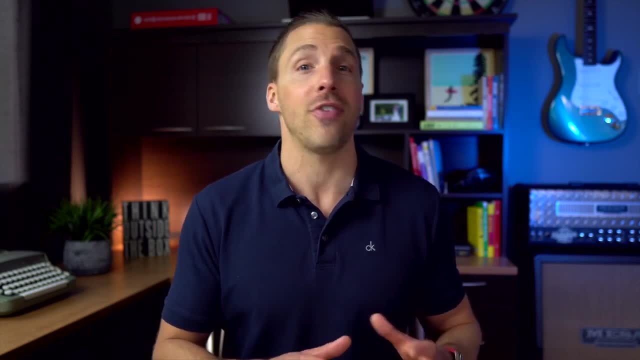 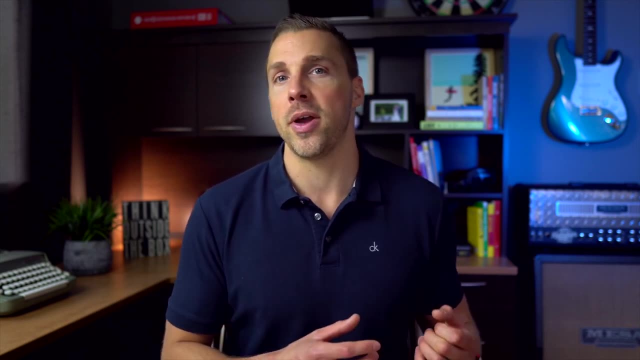 and sort of similarities between those customers to see if you can identify any trends that really make them specific to the rest of the customers. For example, is this group primarily women or is it primarily men? Is it primarily people in their 20s to 30s? 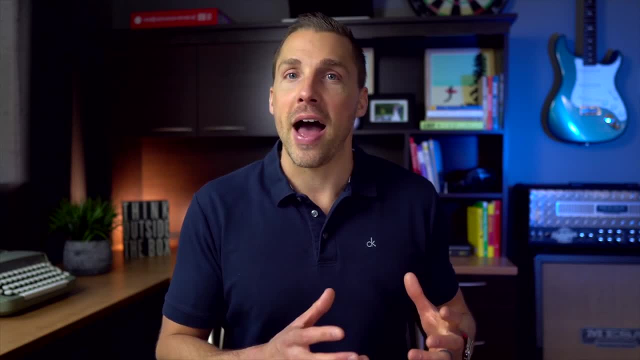 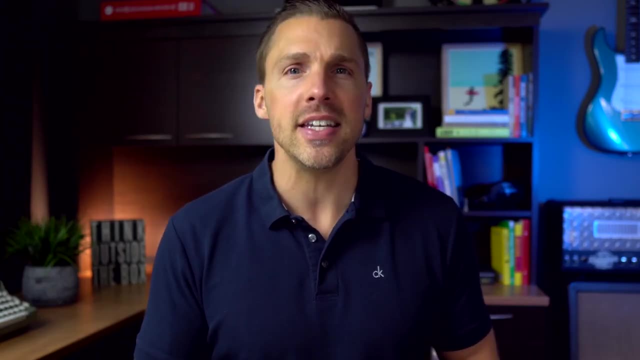 or is it people in their 40s and 50s? Is it people that buy a certain type of product or service, or a different type of product or service? Well, once you have this information, it's time to dig even deeper with something I call customer conversations. 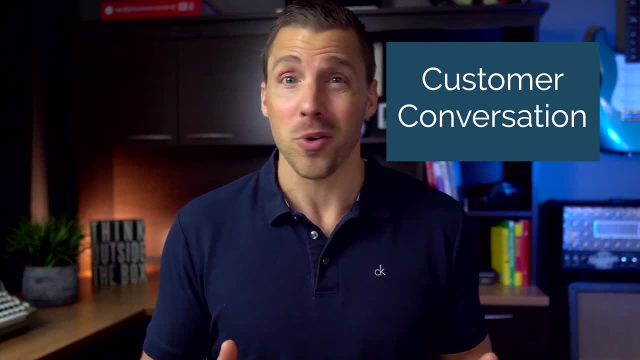 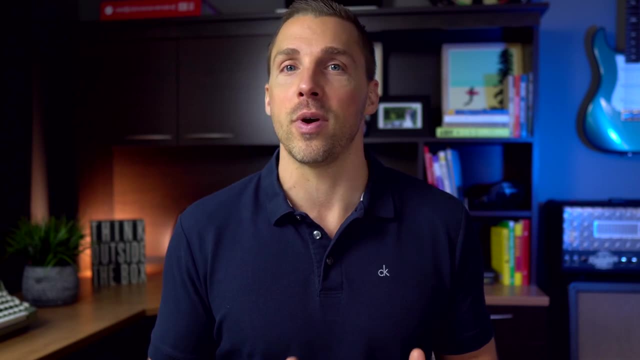 What you wanna do here is pretty much exactly what it sounds Really. just pick up the phone, have a chat with your customers, find out what their problems are and how your business has helped to solve them, and really what they're looking for next. 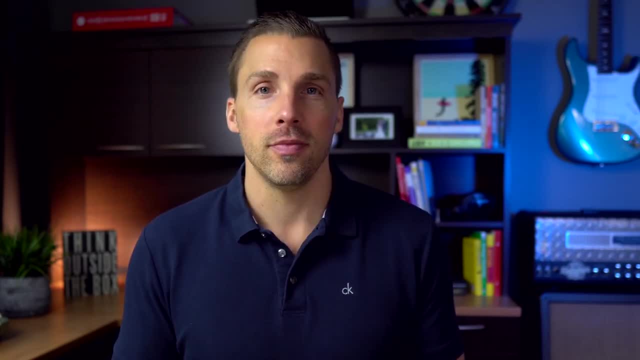 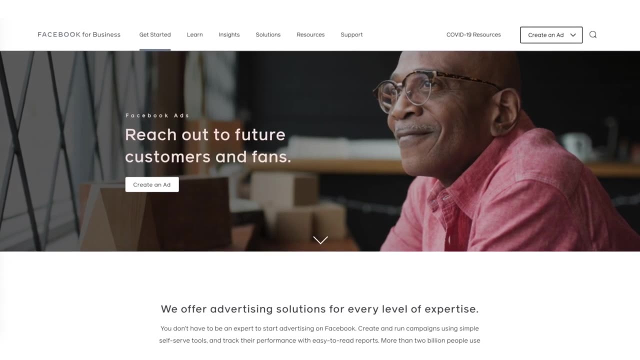 All of this is going to give you incredibly valuable market research. All right. next up, we have Facebook ads. Now, I appreciate this one is not free, but it can be done for very, very inexpensive- as little as a few dollars a day. 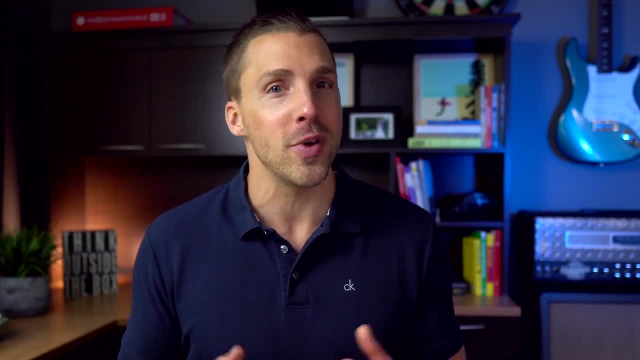 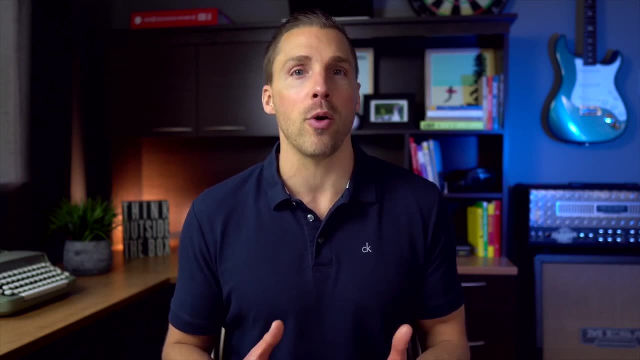 but it can be done for very, very inexpensive- as little as a few dollars a day- and any investment you make here is gonna pay off in the long run by making sure you're doing the right things for the right people. Essentially, this strategy was popularized back in 2007. 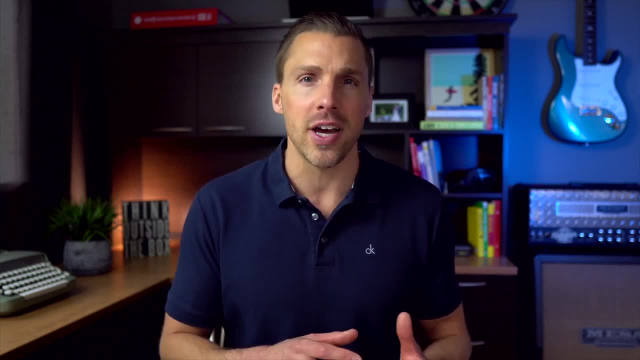 with the release of the 4-Hour Workweek by Tim Ferriss, where he advised using Google AdWords in order to split, test different book titles and different taglines in order to find out the winner. Well, fast forward to today and this strategy is just as relevant, if not more.